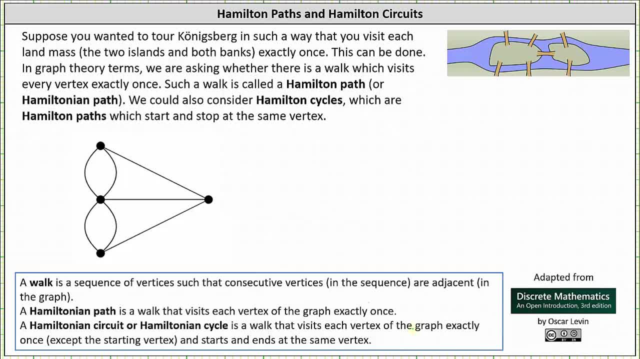 then also determine if there's a Hamiltonian circuit. We can begin with any vertex. Let's start here, at the top, And now we need to form a walk that visits each vertex exactly once, So we can go down to the right, down to the left. 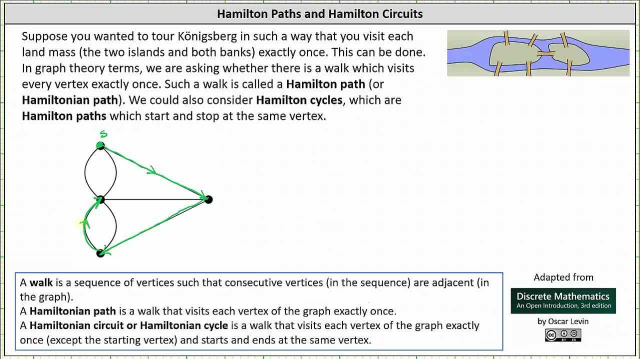 and back up to this last vertex. We can stop here. This is a walk that visits each vertex exactly once. This is an example of a Hamilton path, But also notice: from here we can return back to the starting vertex without visiting any other vertex twice except the starting vertex. This would be. 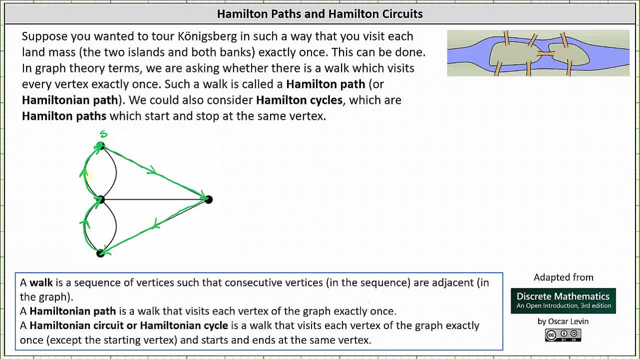 an example of a Hamilton circuit. Let's find a different Hamilton path. Let's say: this time we start over here on the right. If we go down to the left, up and up, we can stop here. This is an example of a different Hamilton path. We have a walk that. 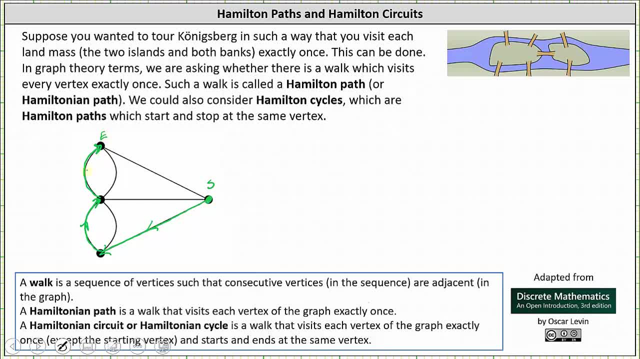 visits each vertex exactly once And notice how I'm using arrows to show the walk. Sometimes you'll also see numbers to show the walk And once again, if we continue the walk, we can go back to the starting vertex without visiting any other vertex more than once. this is an example of a different Hamilton circuit. 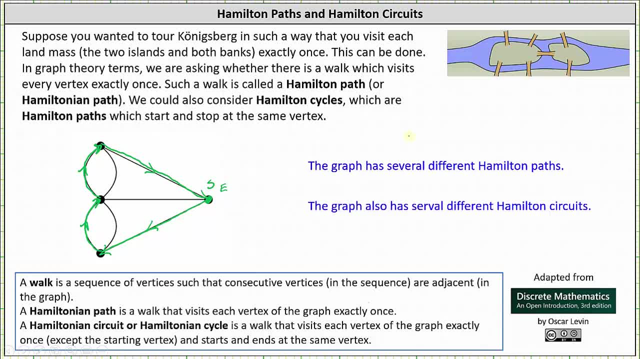 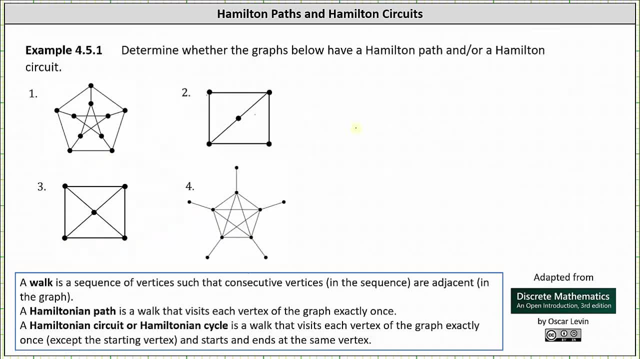 The graph has several different Hamilton paths. The graph also has several different Hamilton circuits, And now let's look at some more examples. We want to determine whether the graphs below have a Hamilton path and or a Hamilton circuit. We can begin at any vertex. 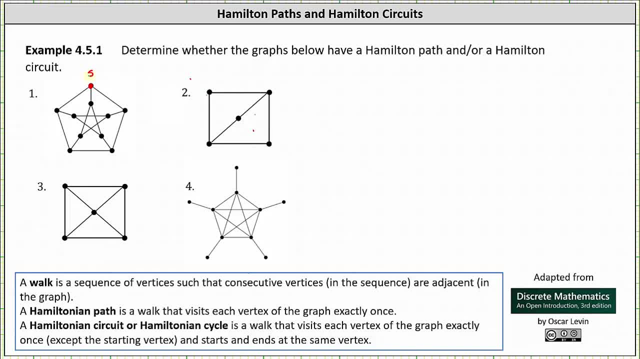 Let's start here, at the top, And now we need to see if we can form a walk. visits each vertex exactly once. Let's go around the outside first. Now we need to go inside. Let's go ahead and go right down to the left. 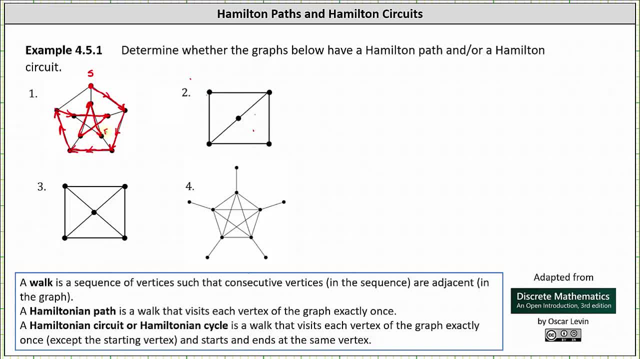 up and down to the right. We can end here. We have a walk that visits each vertex exactly once, and therefore the graph does have a Hamilton path. Notice how we're not able to return back to the starting vertex unless we revisit other vertices more than once. 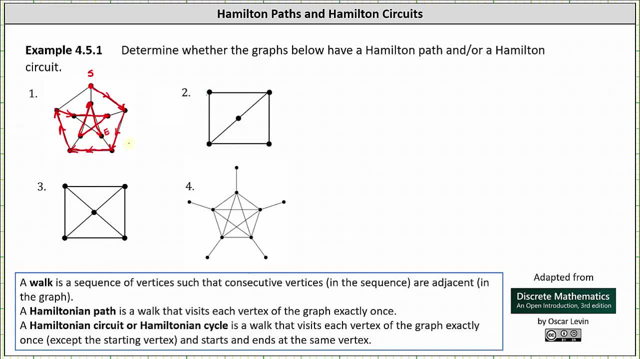 and therefore the graph does not have a Hamilton circuit. The graph has a Hamilton path. The graph does not have a Hamilton circuit. And now let's look at number two. Let's go ahead and start here, at the top. Let's go down over to the left, to the middle. 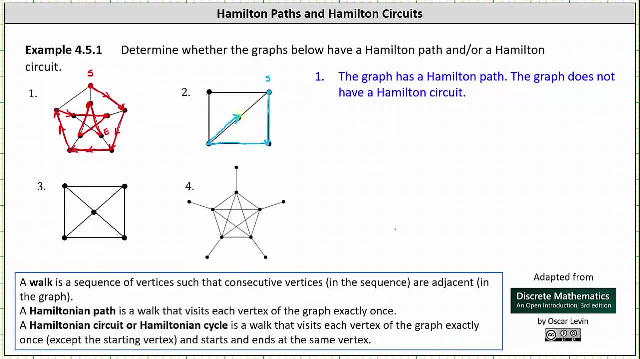 Notice. now I'm stuck. I'm not able to continue the walk without revisiting a vertex more than once, so it may appear as if the graph doesn't have a Hamilton path or a Hamilton circuit, but that's not always true. There may be a different result. 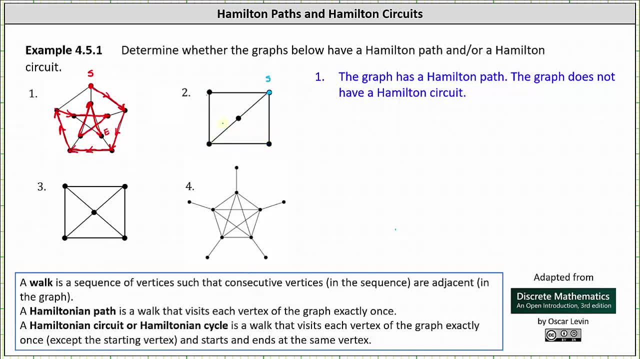 starting from a different vertex. So let's go ahead and start in the middle this time and try again. Let's go up to the right, down to the left and up. Notice, here we do have a Hamilton path. We can't get back to the starting vertex. 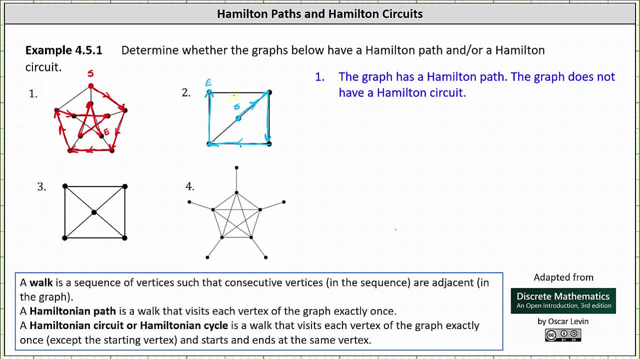 without visiting other vertices. We can't get back to the starting vertices more than once, indicating there is no Hamilton circuit, but the graph does have a Hamilton path, Just because we're not able to find a Hamilton path or circuit on the first attempt. 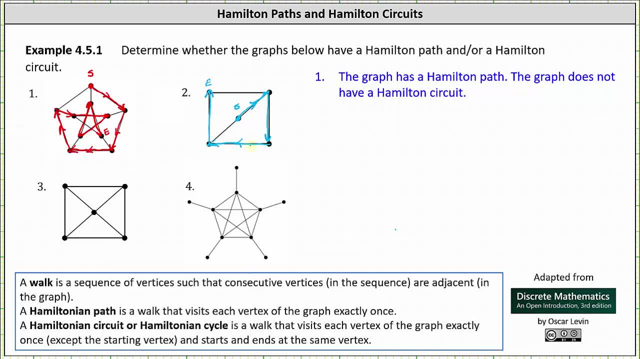 doesn't mean they don't exist. So for number two, the graph has a Hamilton path. The graph does not have a Hamilton circuit. And now let's look at number three. Let's go ahead and start here, in the upper right-hand corner. 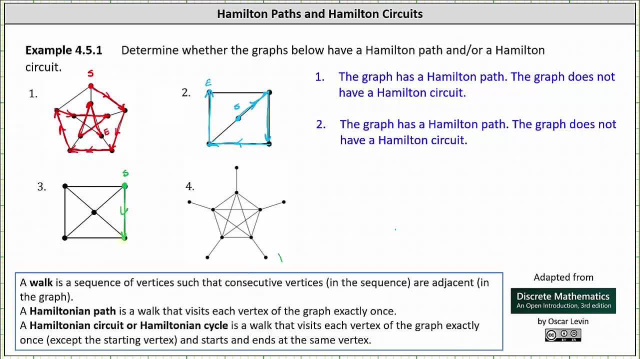 Let's go down To the left, to the middle, back up to the left. If we end here, we have a walk that visits each vertex exactly once, which is a Hamilton path, And if we continue, we can return back to the starting vertex. 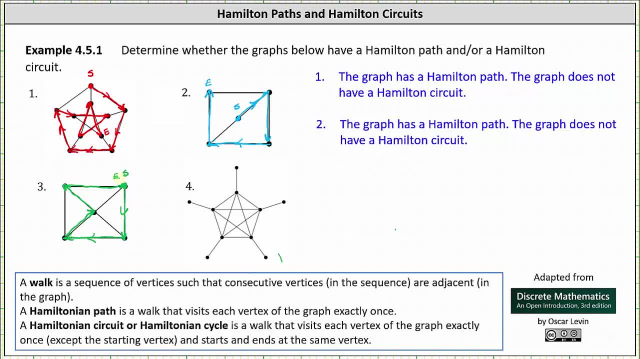 We also have a Hamilton circuit. So for number three, the graph has a Hamilton path, The graph also has a Hamilton circuit And for the last graph, we should recognize something is off here If we start at one of the vertices on the Pentagon. 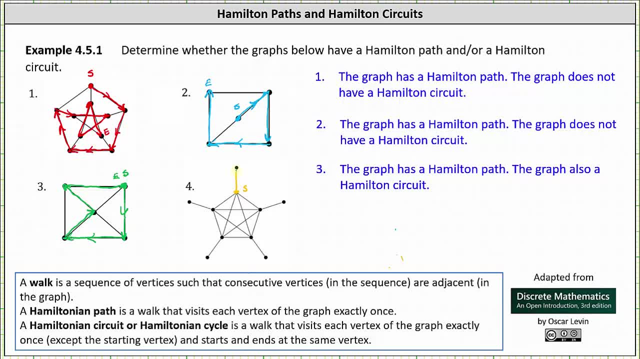 at some point we have to visit one of the outer vertices, let's say here, And as soon as we visit this vertex, we're stuck. we cannot return without visiting the previous vertex more than once, which indicates this graph doesn't have a Hamilton path.